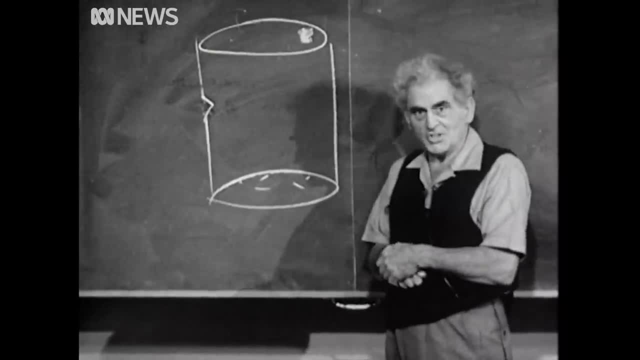 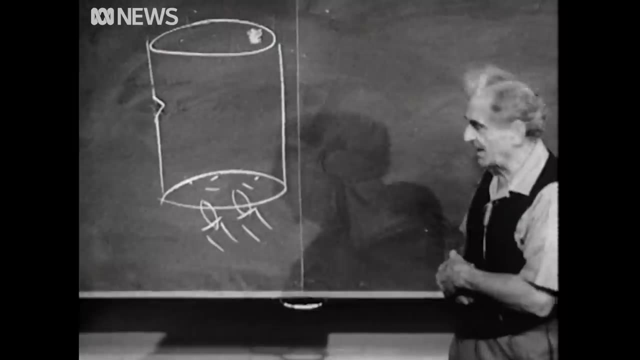 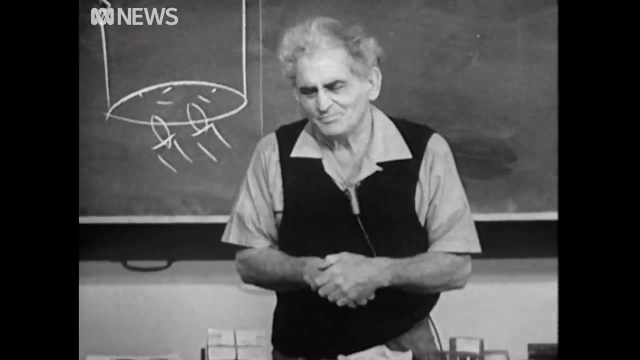 We hope that this is what we hope for. so we are going to do it again. We are heating the water in here, and after a bit I'll go out there and we'll try it once again, because I do not like to- well shall I say- have things fail. Now you know my philosophy. It is important that we subscribe. 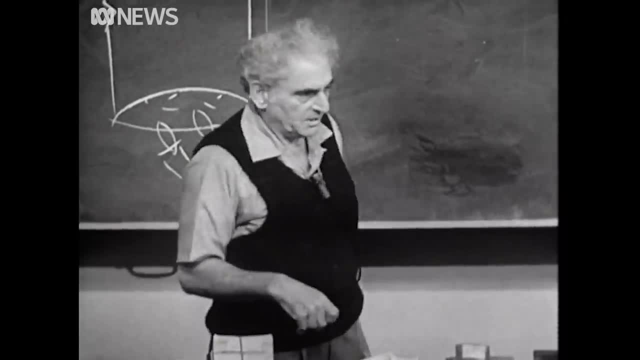 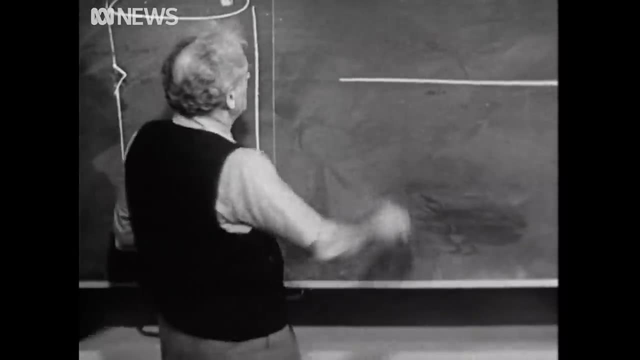 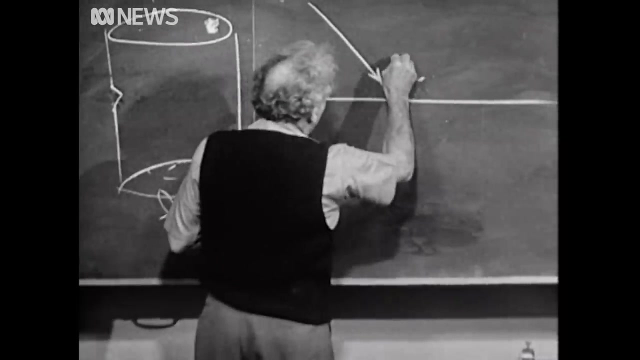 to the requirements of nature While the water is cooking. let's consider another thing. You know that if we have a surface which is reflecting, and we have, say, some energy incident this way, like a ray of light, and we draw a perpendicular to that surface, there is reflection so such that 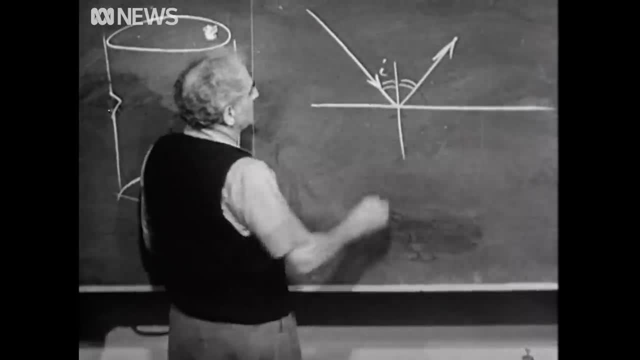 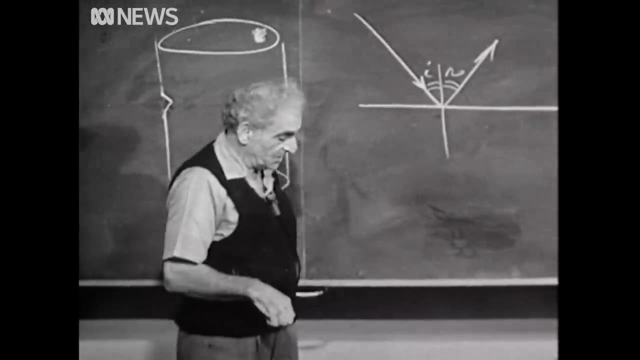 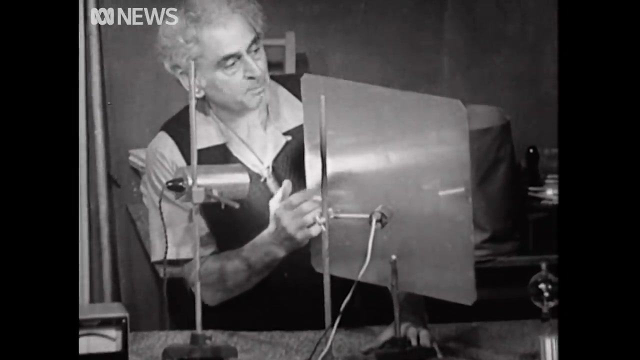 that angle, you know, is equal to that. This is called the angle of incidence. This is the angle of reflection. Now, light energy behaves according to this law, and we have an instrument to show you that. Consider the following: Here is a highly reflecting metal plate. Here is an incandescent. 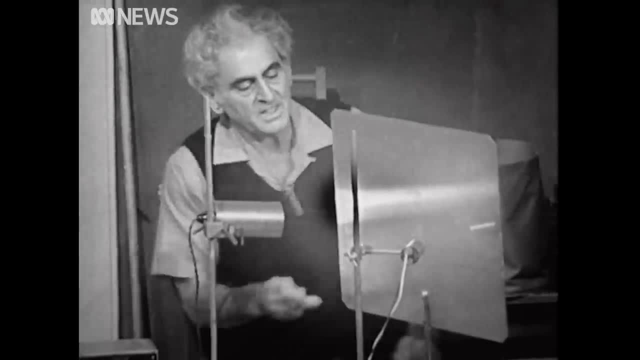 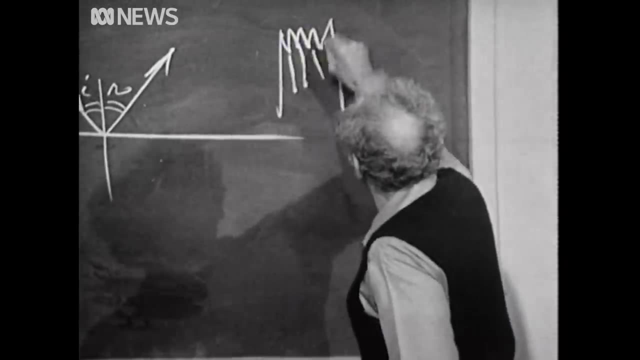 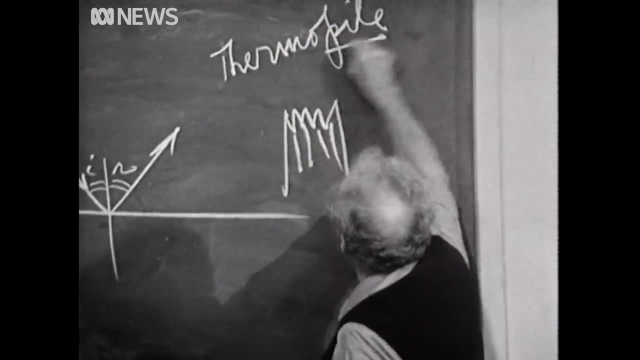 lamp, which I'll just show you quickly, and here is an array of thermocouple junctions. Thermocouple junctions called a thermopile. See it: Thermo pile, a pile of thermocouples. Got that. Now we are going to put some radiation energy from this lamp. 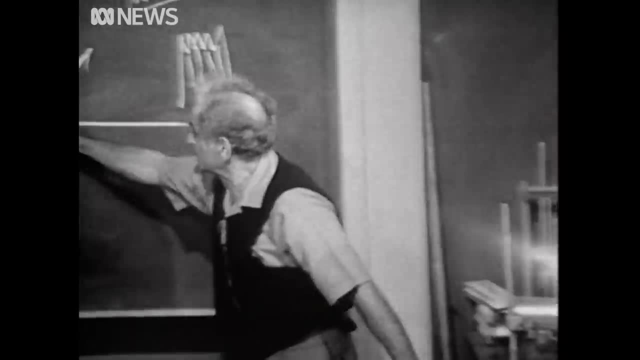 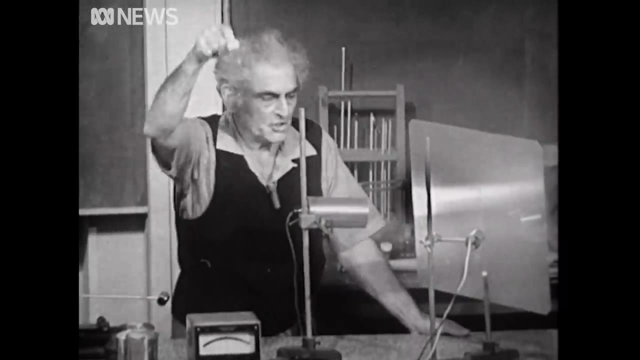 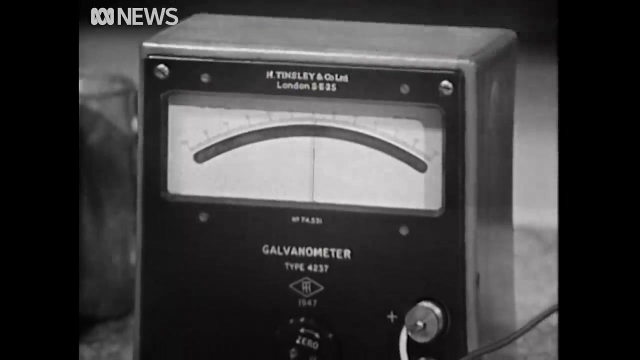 on this plate, It will suffer some reflection according to this law. This thermopile will pick up the radiation electromagnetic, convert it to thermal energy and here we have a zero center meter which I hope shows when I have made the right angle. the 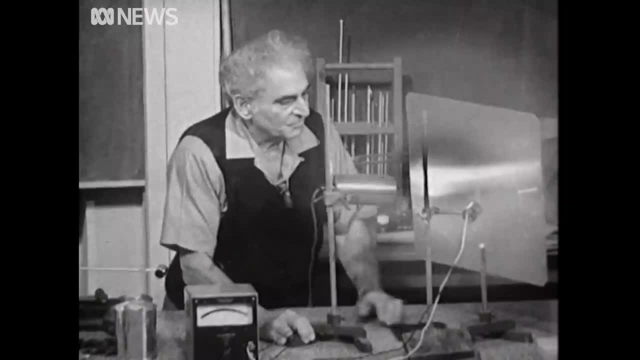 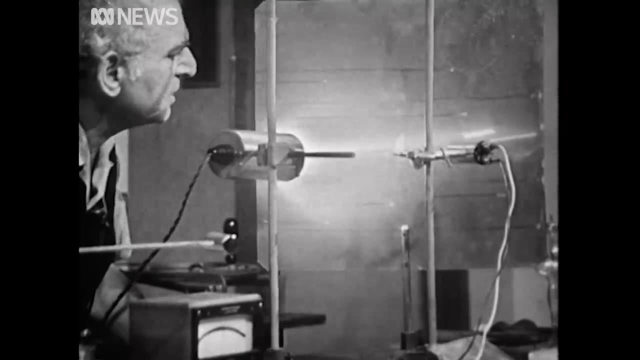 correct angle, equal to the correct angle. Watch it now. We'll just have to see this and then the meter. Oh, I don't know how you'll do it, but we need to see the meter too. Watch it, I'm bringing. 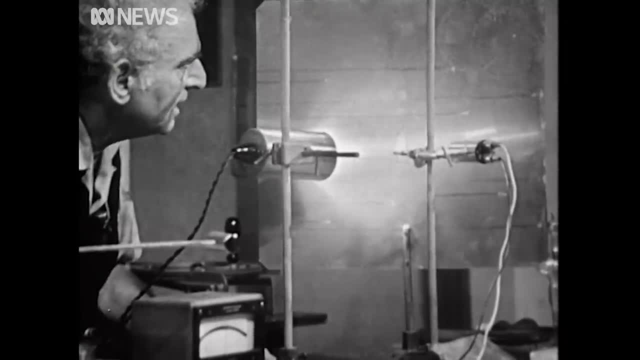 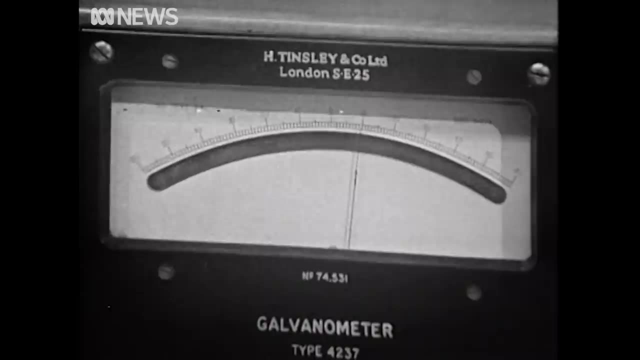 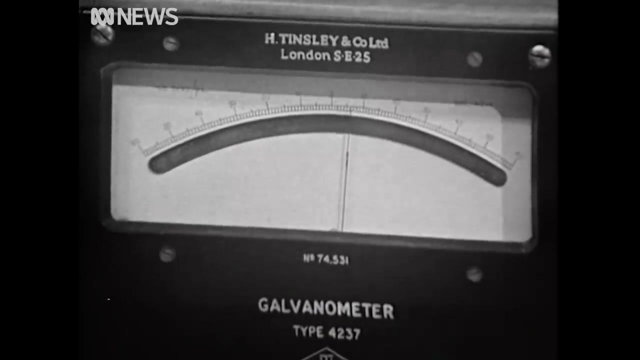 it in, I'm bringing it in. I can't tell when the meter is reading. Is it reading, Yes, yes, Now watch, I'm going to go away from that angle And now it's coming back. Now it's coming back. So a wonderful demonstration. 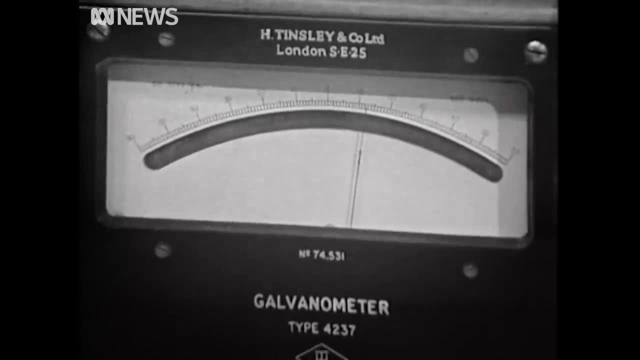 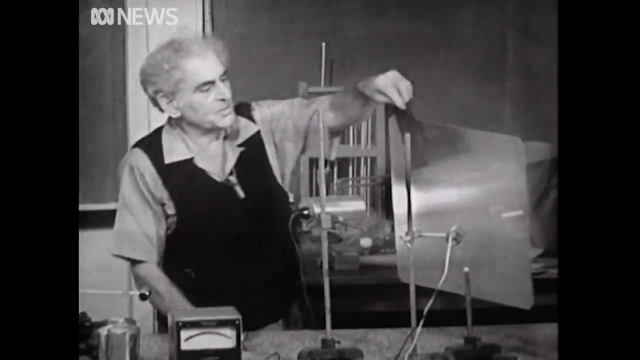 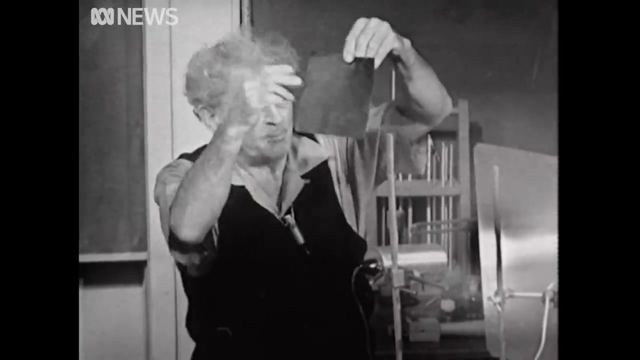 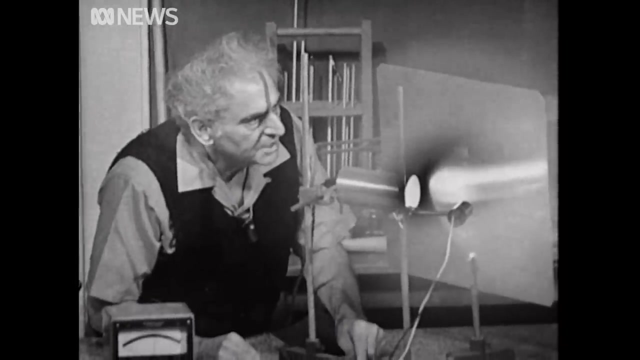 There is a best angle. There is a best angle. Now let's do it all over again, and this time intercept the energy, Not with a shiny reflecting surface, but a highly absorbing one, a black piece of paper. Let me come back to the angle which gives us the best energy received by the meter. 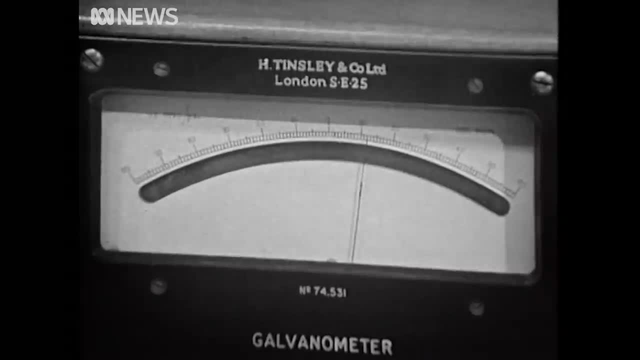 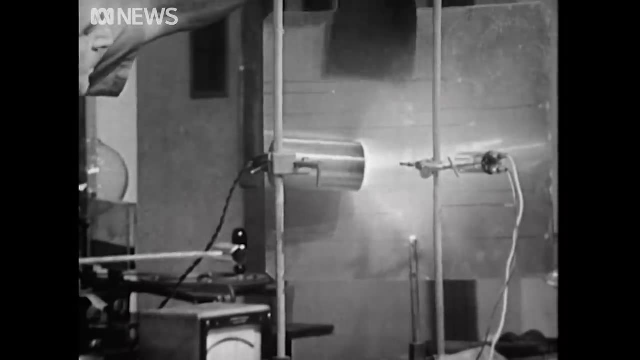 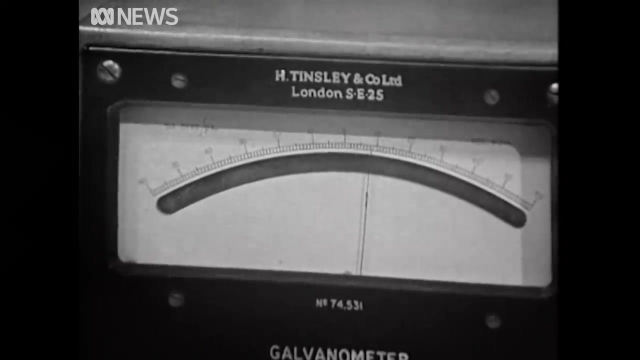 I can't tell. I have to see the meter. Is that it All right, Now I'm going to interpose that piece of paper. Watch the needle now. Watch the needle now. Do you see it's going back. It's going back, Showing that very little energy is being. 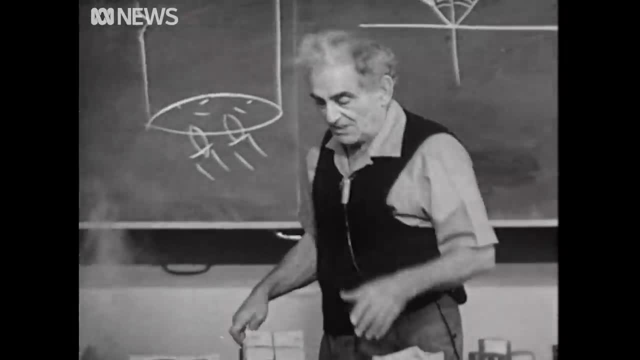 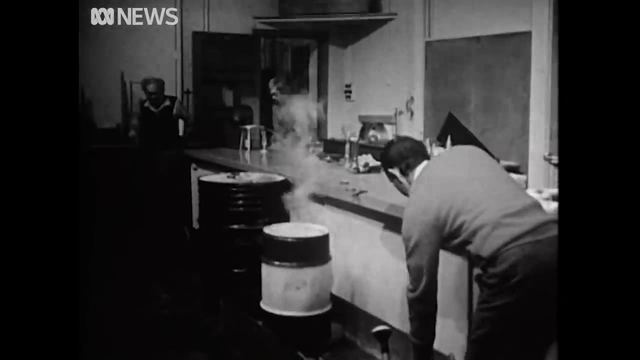 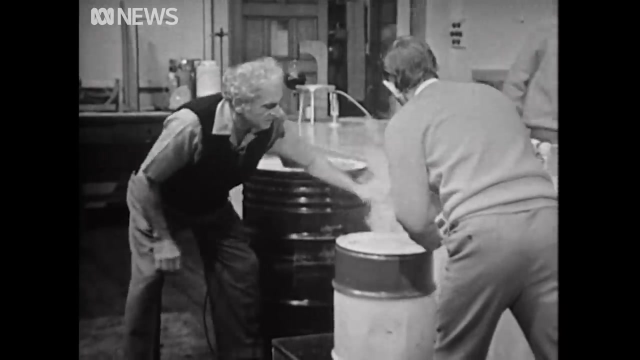 reflected Very good. That tank out there is boiling now beautifully. Let's try it, Because I feel like Otto Von Garrycki making a demonstration. Josh, can you switch the gas on? Yes, but don't switch it off yet. Now switch it off. 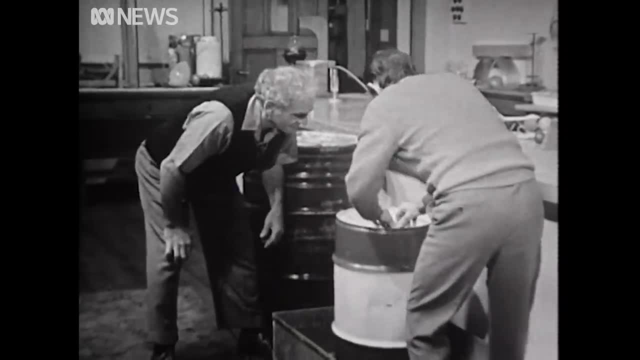 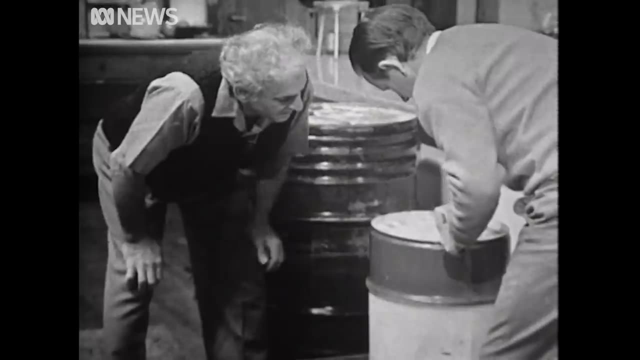 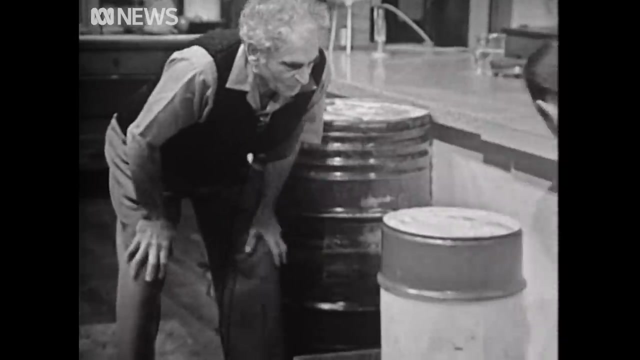 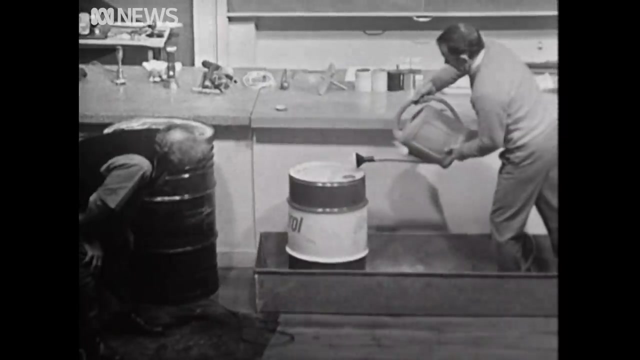 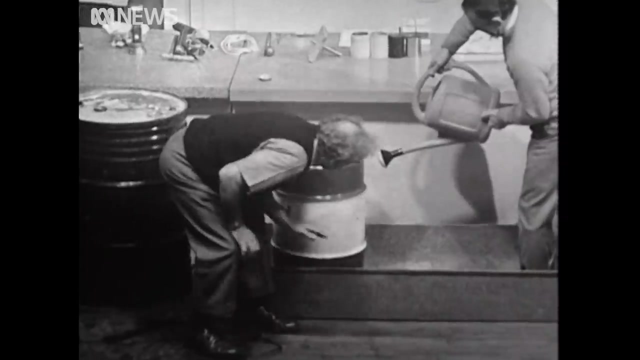 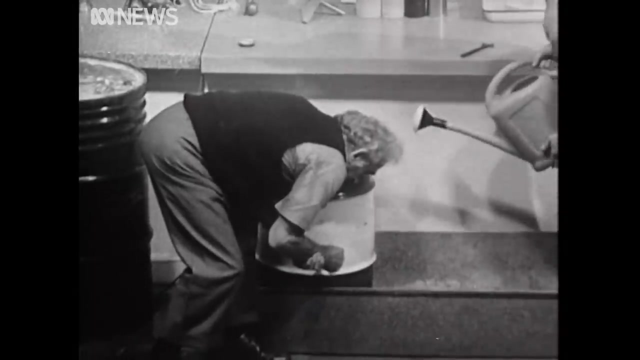 Plug it up, up, Mache schnell. If we lose any More tight, Watch it. Anderson is going to be drowned. Easy, Easy, Hold it, Hold it, Hold it. Let me hear, Oh, the water's boiling feverishly inside. 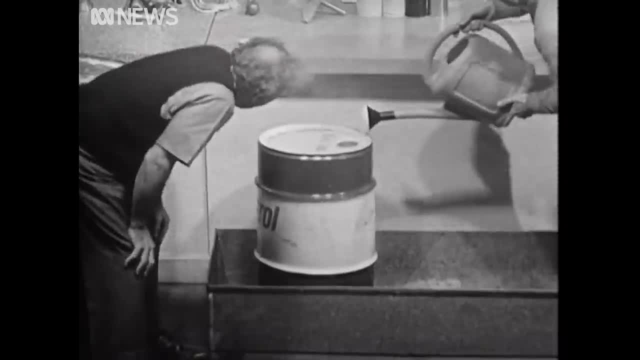 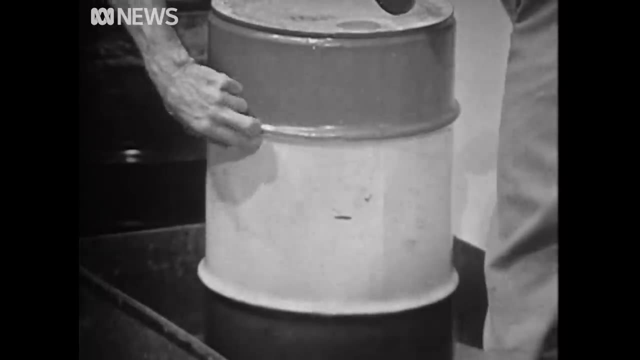 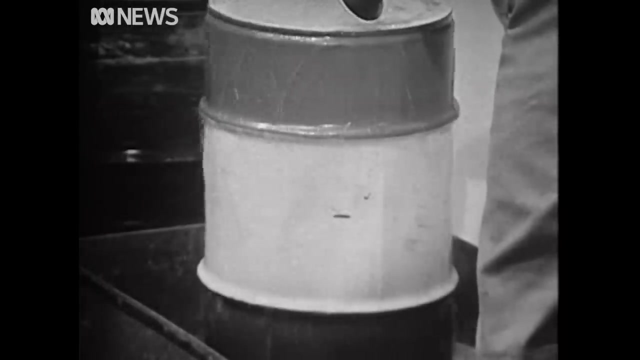 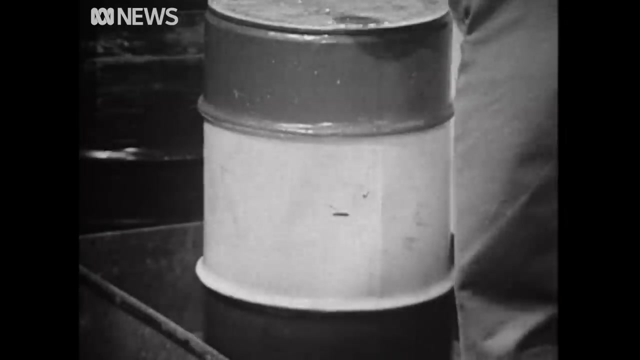 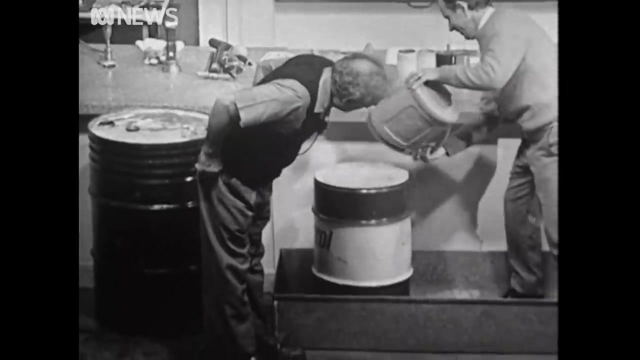 The pressure is very low. But it appears again that this tank is too firmly reinforced with those ribs, those circular ribs, Anderson, and it will not go. No, we are lost. Anderson is resorting to some ice. We are in desperation and in despair. 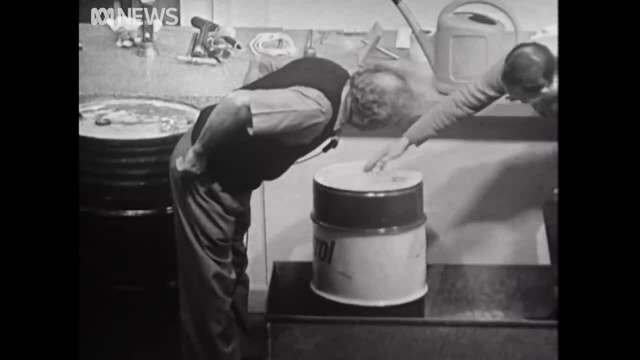 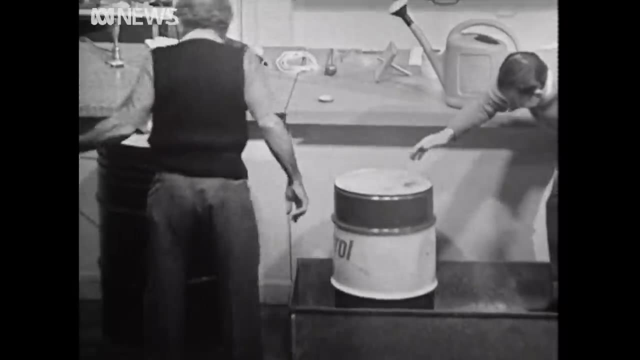 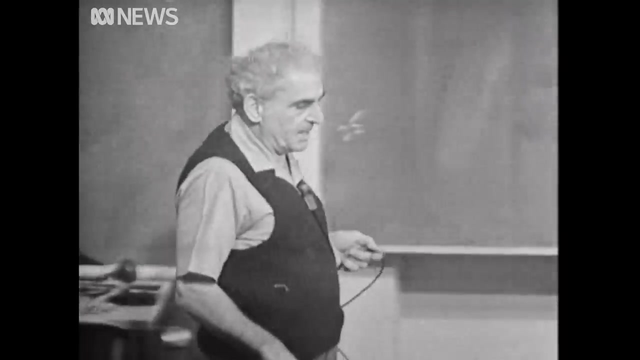 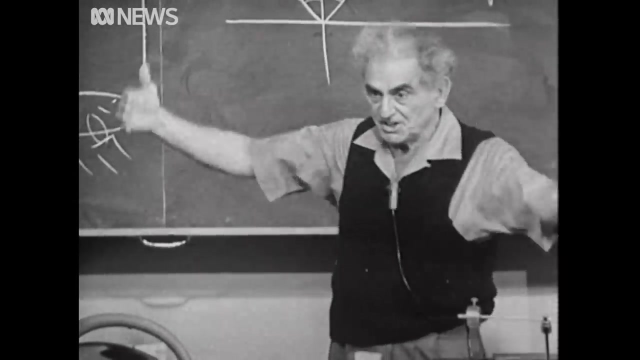 If it does go, we'll get drowned. Nature has thwarted us again. Yeah, Let us abandon it, Anderson. It is too bad, But I had hoped to see it, And I'm reminded that I tried to do this in Uppsala, Sweden, with a huge tank made of Swedish steel and 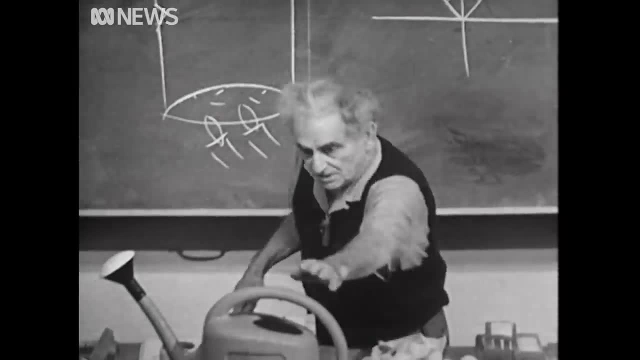 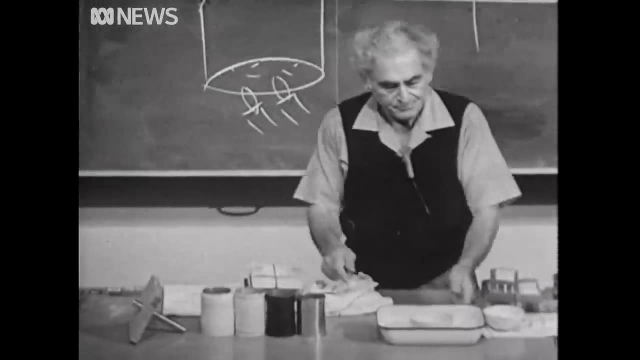 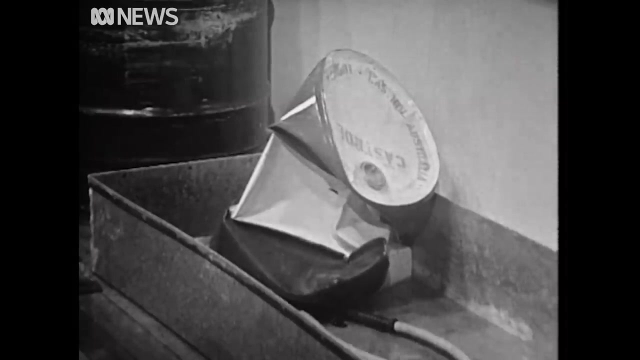 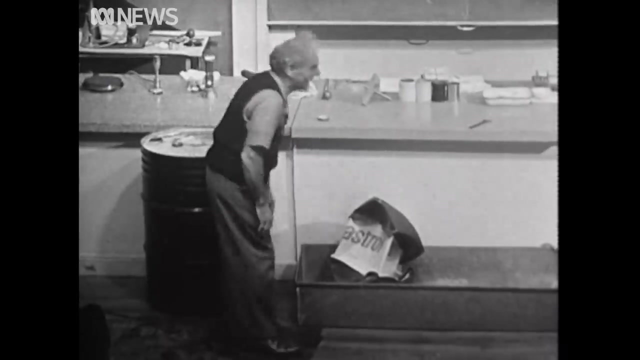 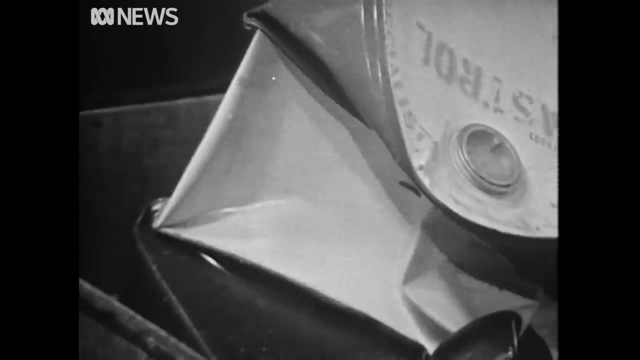 it would not go. So I said Swedish steel is too much for us. So a little now, aside Problem It went, It went, It went. Ho ho, It went, Ho ho man, Oh, it went, It went. Ho ho, ho ho. Oh, mamma mia, Did it go. Oh, did it go. 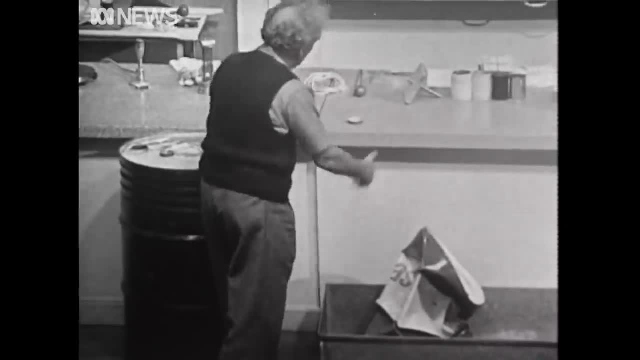 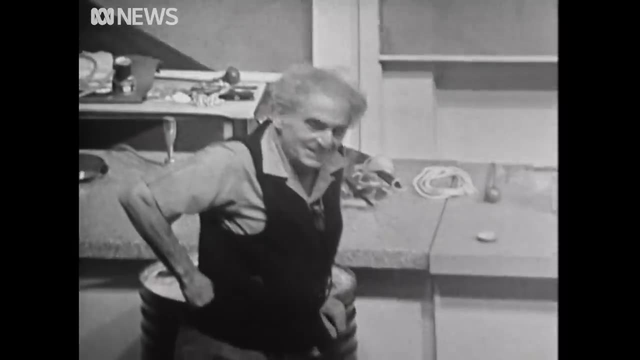 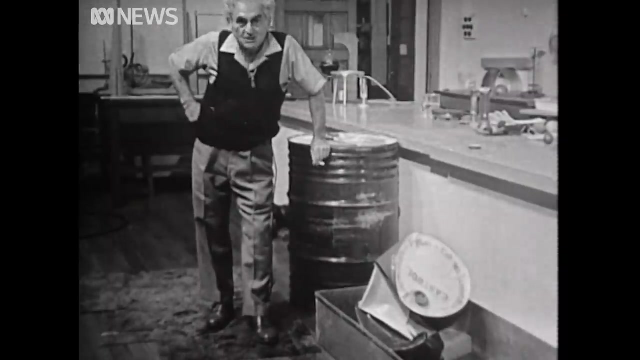 Oh no, Oh no, No. Well, ladies and gentlemen, we did that right up. smart, didn't we Beautiful? I had given it up. I had given it up. Was this caught on camera? Was it? Well, you were on. 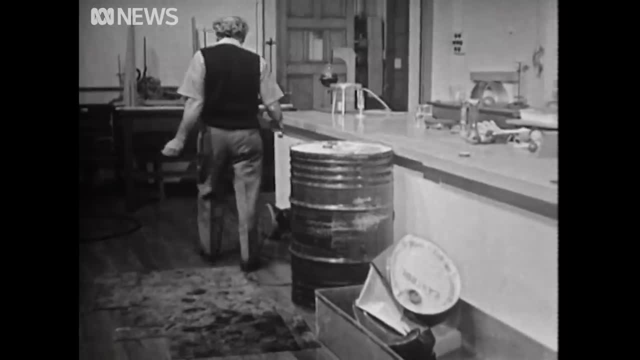 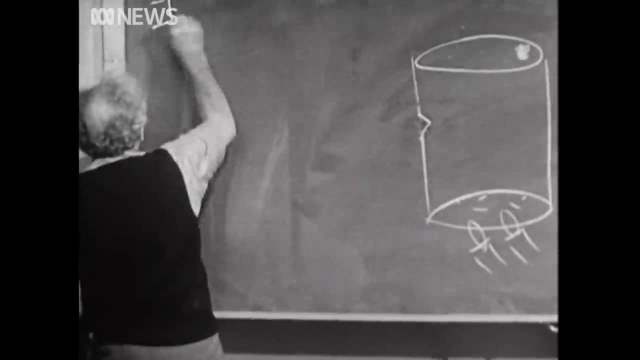 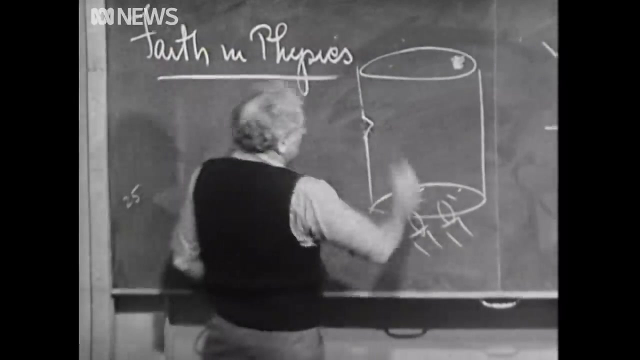 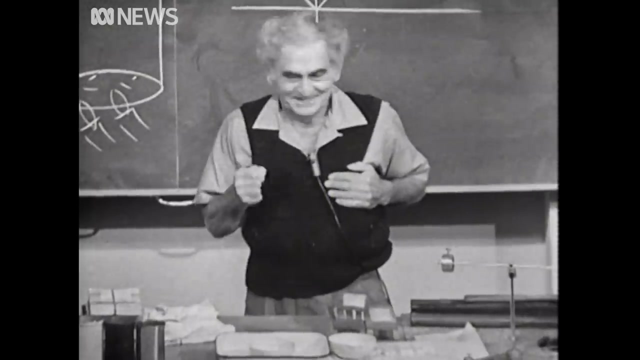 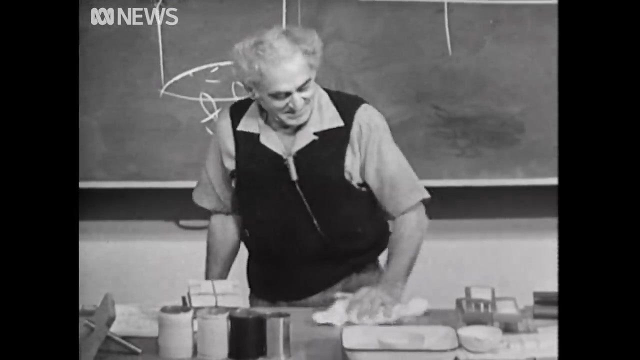 it. Oh, mamma mia, I am ready to dance for joy. Faith in physics? Huh, Faith in physics. Faith in physics. Yup, That's it. Faith in physics. Oh, that was wonderful. Phew, Oh, this is going. Oh, mother of mine, This is Oh. Now, when I get my composure people. 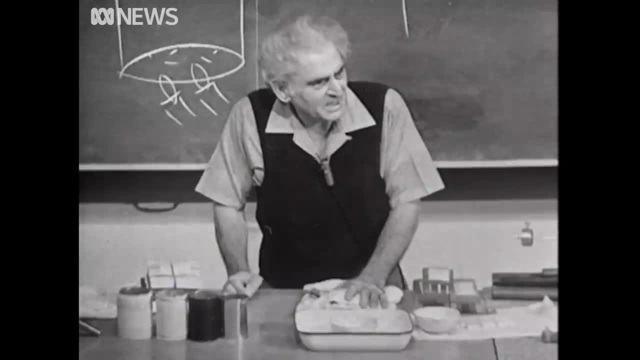 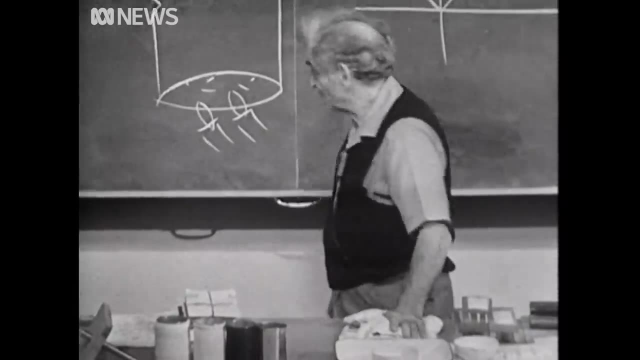 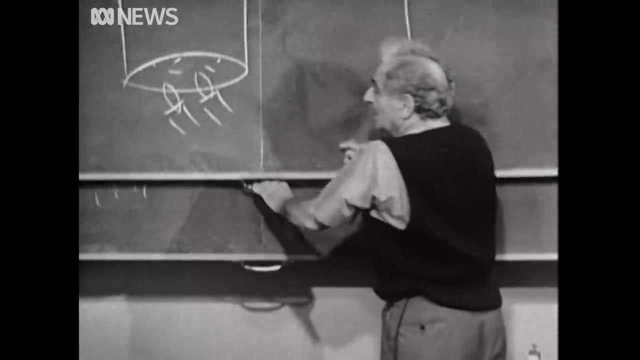 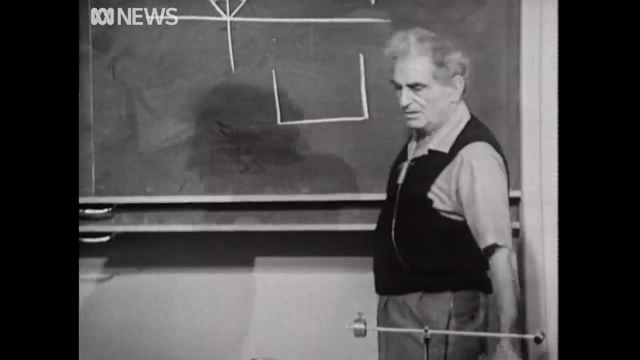 we can return to the program. My great regret is, of course, that I didn't see it. Oh, I missed that. We shall have to do it again, Right? Well, anyway, consider the following A little exercise for you to think about. I have a vessel, not a square edge like that. 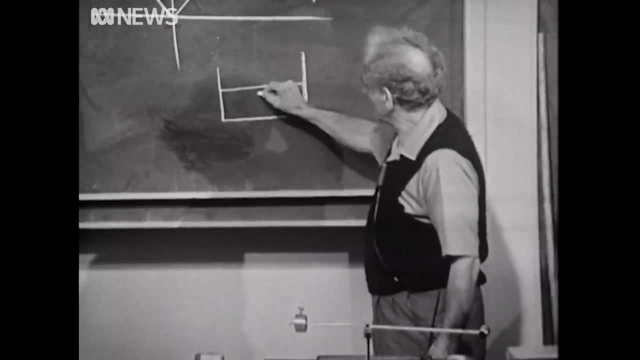